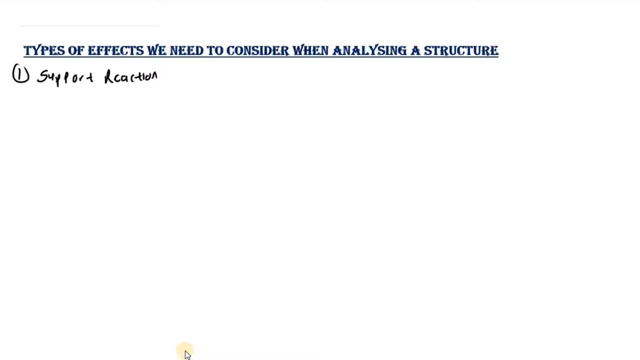 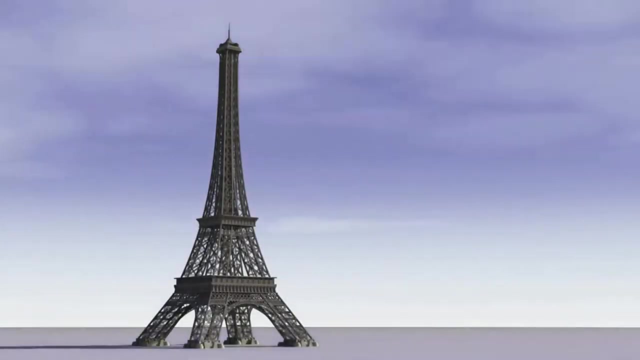 structure stable on the ground. the second is the internal forces or the resultants. now we need to determine the internal forces or the resultant inside the members. for example, if we have a truss, we will need to know the forces inside the truss, like the compression and tension. 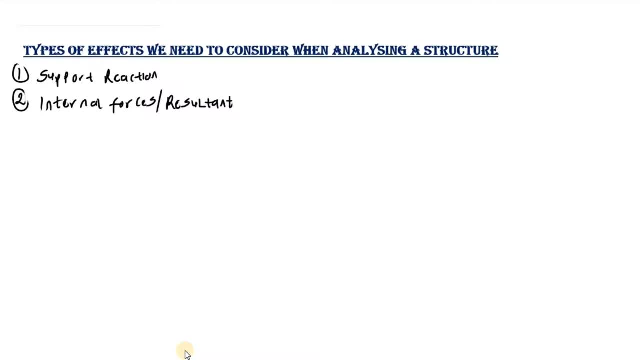 forces for other members, like beams, columns, slab. we also need to know the azia forces, shear forces and the bending moment that will occur due to the member being subjected to load. lastly, we need to know the structural deformation. we need to know the structural deformation. that is how the structure will deform, because any 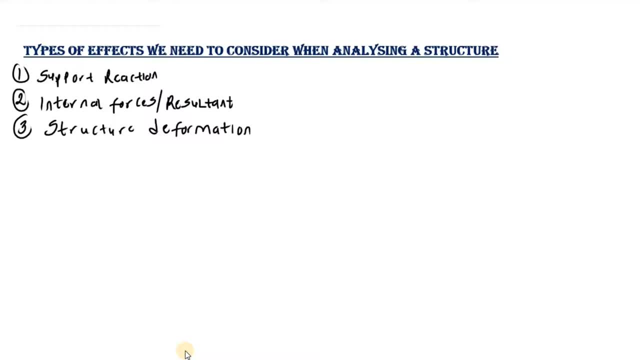 structure we apply a load to will deform, so we need to know how much it deflates and also how much it rotates. now, what do we mean by the load which the structure will be subjected to? there are primarily two categories of load: a structure we experience. the first category is 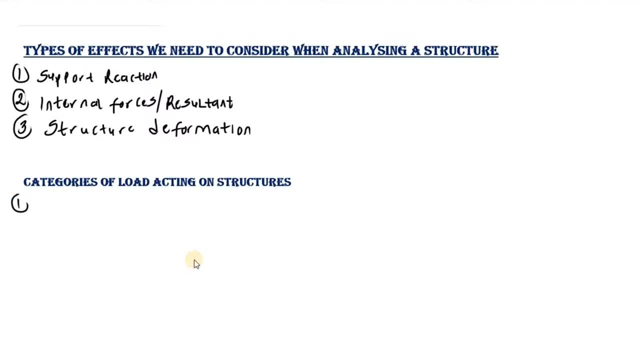 the gravity load. this load we add up and down with the direction of the structure of gravity, and there are two types of gravity load. the first one is dead load. now, the dead load, this would be the self-weight of the structure. that is the concrete we use for. 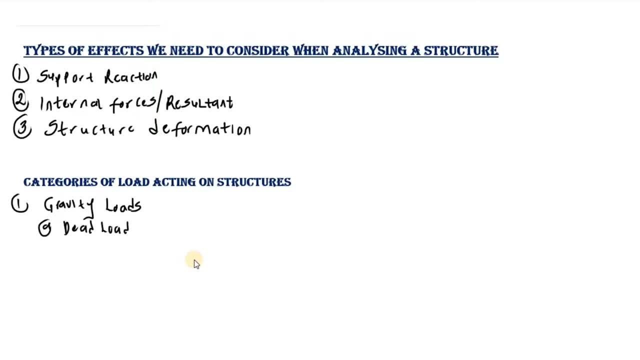 building, the structure, the steel. basically this is the component of the building that is not moving, like the slab, the beams, the the, the columns, the gathers, the shear walls, etc. so these are the dead load. then the second type of gravity load we have is life load, so basically these are also called occupancy load. there are loads that move around in the structure.